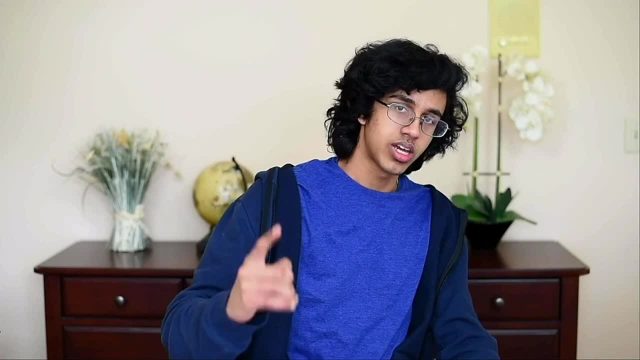 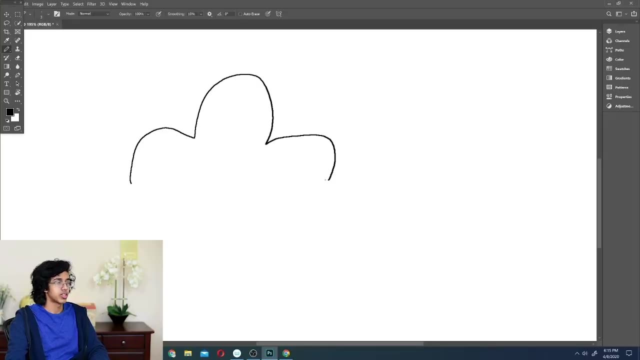 And what does taking the derivative mean? That is right. it is the instantaneous rate of change of a function. So if we take that example of your car right, Let's say you're driving along in your beautiful sedan that looks exactly like that. 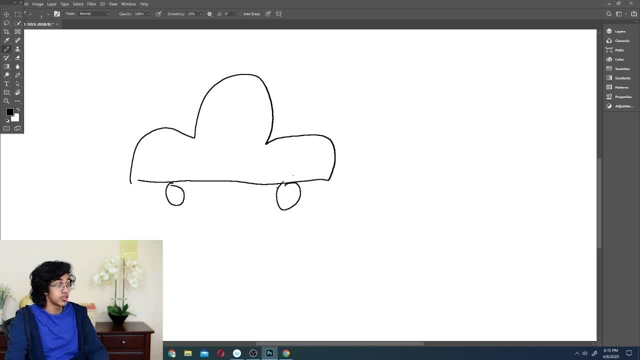 It doesn't even have wheels. I'm just kidding. it has wheels that are under the car name. But anyway, the point is: you're driving along in your car, right? And what is an example of instantaneous rate of change? Okay, so well, we know that your car is moving along, right. 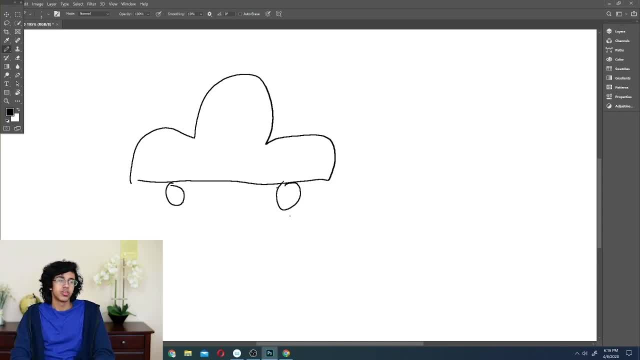 And the rate at which its position changes is called So like average speed. you guys probably know all that nonsense where you take your total distance divided by total time, But we care about instantaneous, because that is what a derivative is. In fact, this is so important I'm going to write it down. 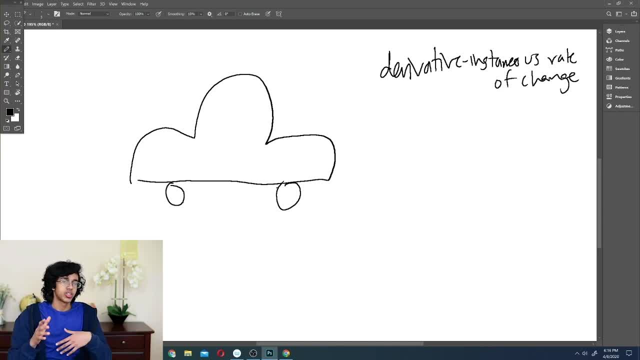 So for a car, our derivative is not our average velocity. okay, You can't just take the total distance over the total time, It is the velocity at a certain point. So whatever your speedometer reads right, Like it says, you're going at 60 miles per hour. that is the derivative of your position. 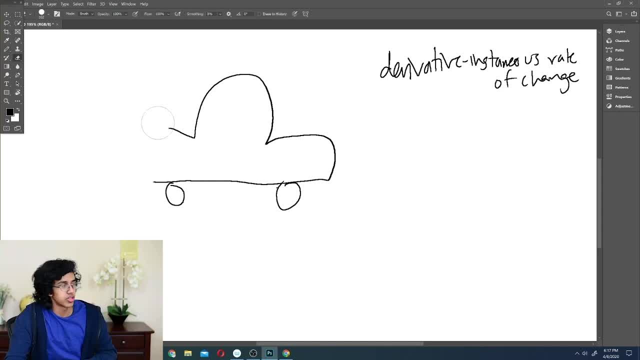 Or in other words, the instantaneous rate of change of your position. So if we think about this in a different way, right? Let's say we have a graph of a function and it basically goes like that: The instantaneous rate of change at every single point is the same, right? 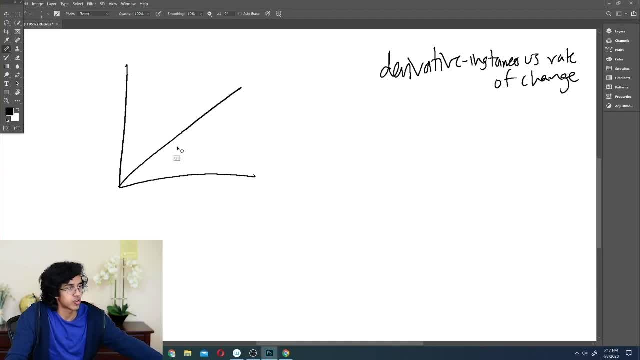 Because your rate of change everywhere is just a slope. But what happens if you have a curved function? right, Then what's your instantaneous rate of change? here It's basically the tangent line, And then that gives you the instantaneous rate of change at that certain point. 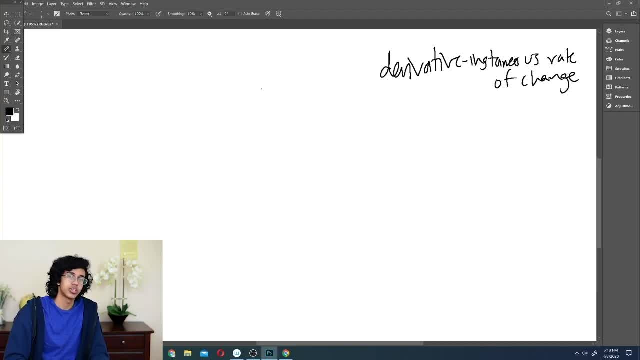 Alright, now there's two notations, because Newton and Leibniz were trolls and they didn't decide to agree on anything, So we got two different notations, But let me just put it out there: Leibniz is superior, okay. 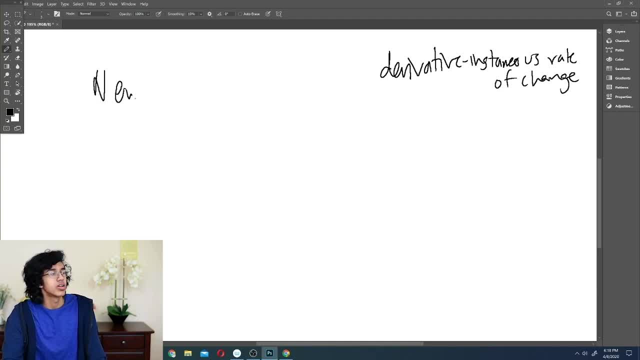 I don't care that Newton knows how to let apples fall on his head, but Leibniz is still OP. So Newton's notation is basically: if you want to find the derivative of f of x, you take the derivative, you just put a prime there. 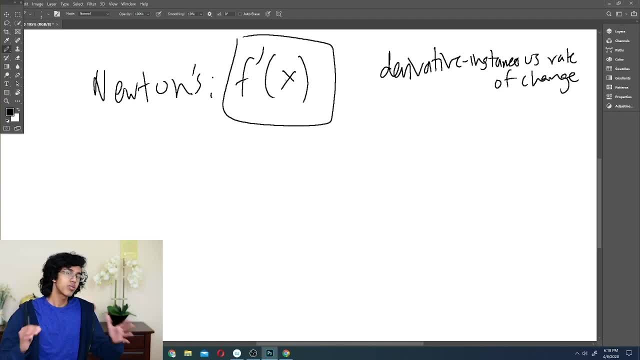 And this represents the derivative of f of x. The only problem with this notation, the reason why it sucks, is because it doesn't tell you anything about the derivative right, Like if you get further into calculus you know that there's, like, other types of derivatives. 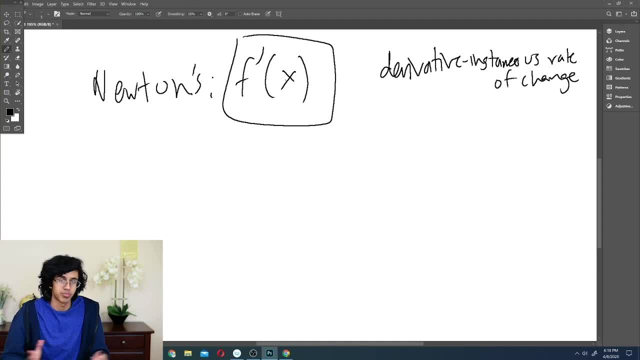 They're not just like you take the derivative of a function straight up. There's like implicit differentiation, there's all kinds of stuff. So this is kind of useless. It's only useful when your function only has one variable. Then we got Leibniz, my boy Leibniz. 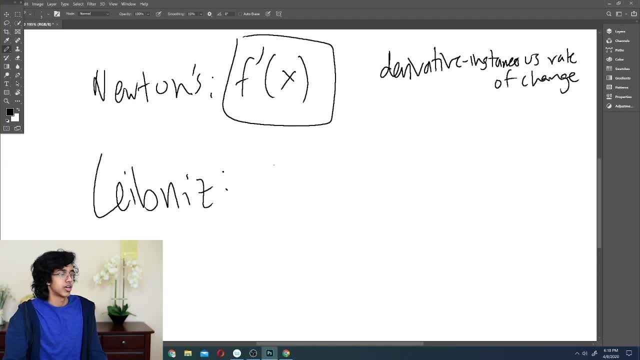 And his thing is: if you have a function like y is equal to f of x, then you write that your derivative of f of x is basically dy over. df is equal to f prime of x Noice. I don't know why I used Newton's notation to explain Leibniz. 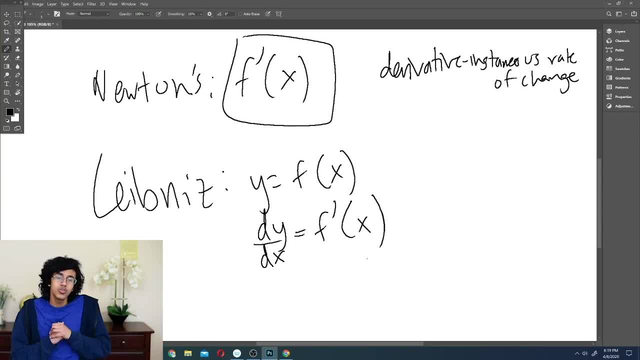 Maybe Newton is superior, but that's not the point, Don't worry. just know that there are two forms in which to write derivatives. Okay, so let's talk about what exactly a derivative is, right? So let us first talk about average velocity, right? 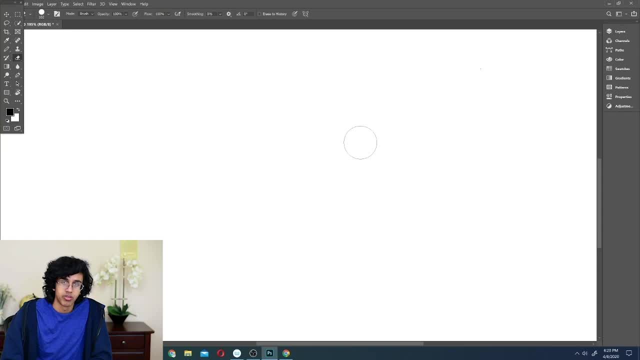 So we're going to be using the example of velocity a lot, because it's basically just the derivative of position, right With respect to time. So if we drew our graph, we basically draw our position versus time. graph x and t. 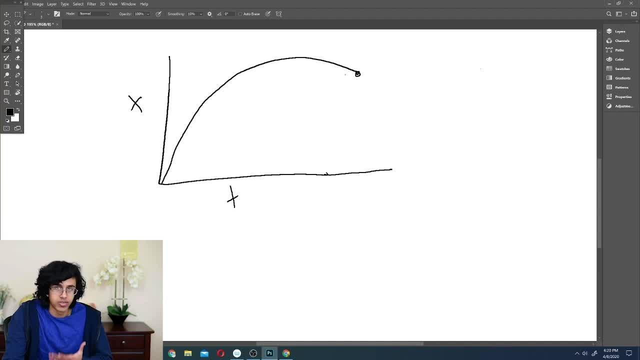 And let's say you go like that. Okay, so we wanted to find your average velocity, right. You take your final displacement minus your initial displacement over your total time, In which case it's like Delta y over delta x, So it's like the slope of this line over here. 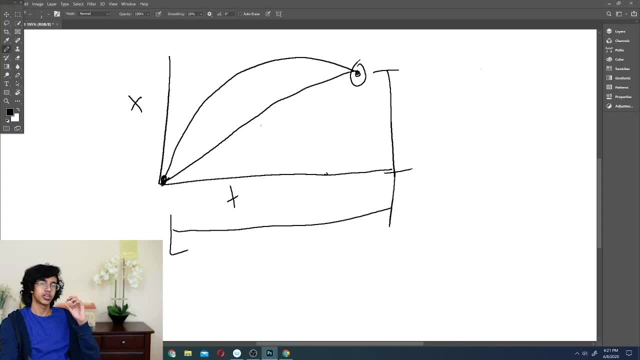 That's a line, okay. Now, this line over here is called a secant line because it connects two points on the curve. But why do we want to define the like velocity at a single point, Which is what we want to do with derivatives, right? 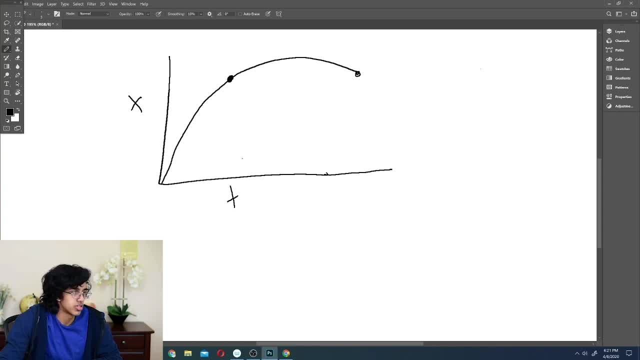 Let's say we want to find it at this point over here. So, like, the average velocity between this point and this point is just the slope of this line over here. right, We already figured that out. Why do we find the average velocity between these two? 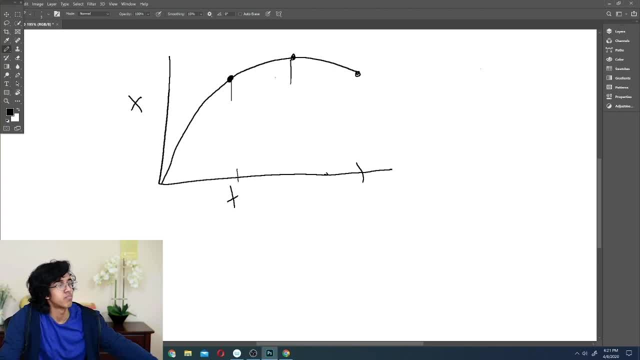 Why do we find the average velocity between t1,, let's say, and t2 over here? Then it would be the same thing, the slope of this line over here, And as we keep bringing this point closer and closer right, Eventually they'll be the same point. 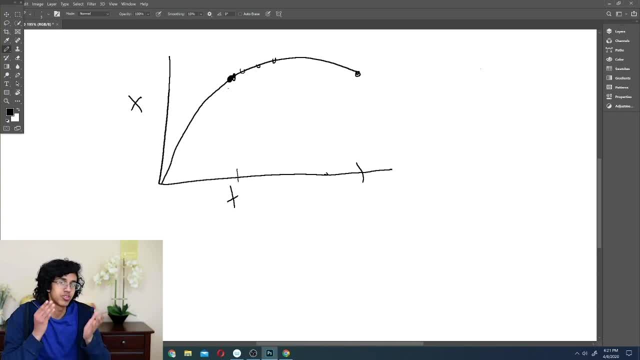 In which case, when we take the average velocity of the same point, it's just the velocity at that point, And then we get the derivative. So basically, the derivative is when you shrink the secant line until the two points are touching at the point that you want to take the derivative of. 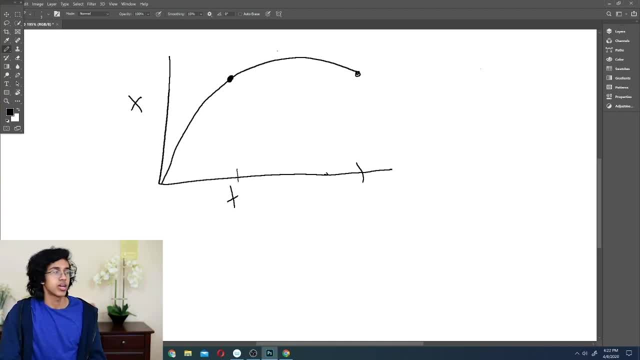 Okay, so first things first. how do we find the slope of the secant line? Let's say this is t1, x1, and then this is t2, x2, right, Then the slope is just going to be delta y, which is x2 minus x1, over t2 minus t1. 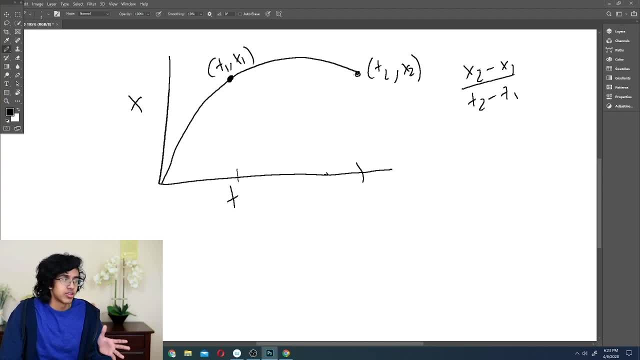 Okay, so we want to define the derivative right And we knew that the derivative is just the limit of the secant slope as we bring the other point on the secant slope all the way back to the first point. So we could basically say that the position of the function of time right 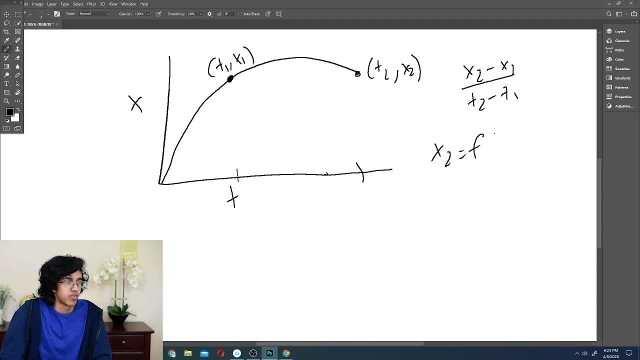 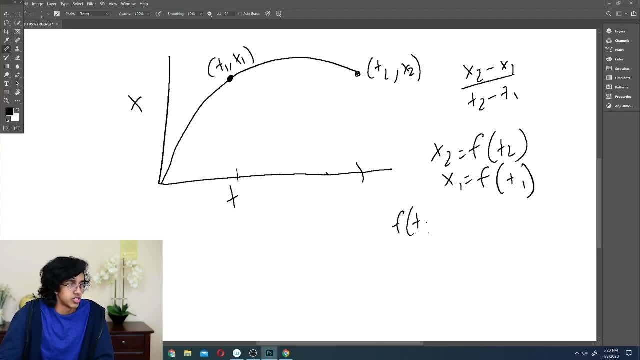 Okay, so the slope of the secant line is going to be f of t2 minus f of t1, over t2 minus t1. And we want to take the limit as t2 approaches t1. So they get really close and then once they're one point, that's your tangent slope. 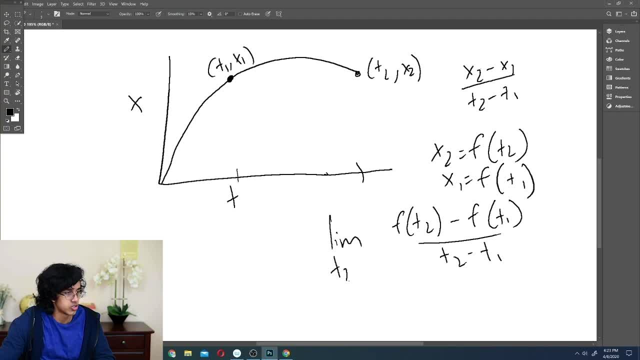 So we'll take the limit of this as t2 approaches t1. And you can think of t1 as a constant. So this, right here, is the first definition of a derivative. Now you want to know this equation because, like on the AP exam, 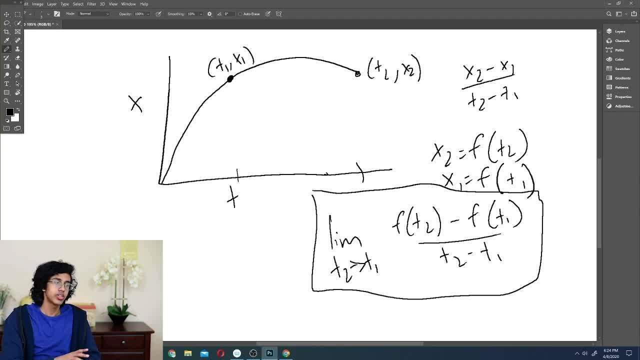 sometimes they give you a slightly modified version of this and they ask you to give it in terms of the derivative Like. sometimes they like to just randomly put a 2 over here, right, So now you have a 2 times this. 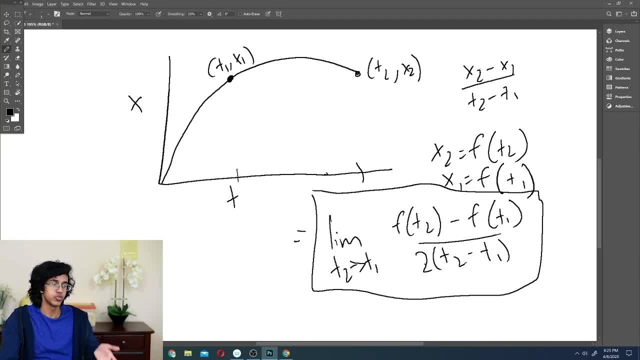 So if this inner part is just equal to the derivative and you put a 2 in the denominator, then what is it? It is one half of the derivative at t1.. So just don't get trolled by that. This happens on the AP exam. but let us figure out what the other definition is. 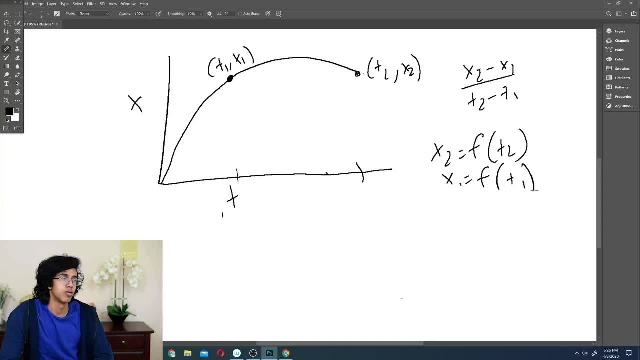 because they also use the other definition of a limit. So one way to bring this point closer to the other point is to obviously just change t1.. Change t2 to t1, right. But what happens if we just set this distance over here to h, let's say: 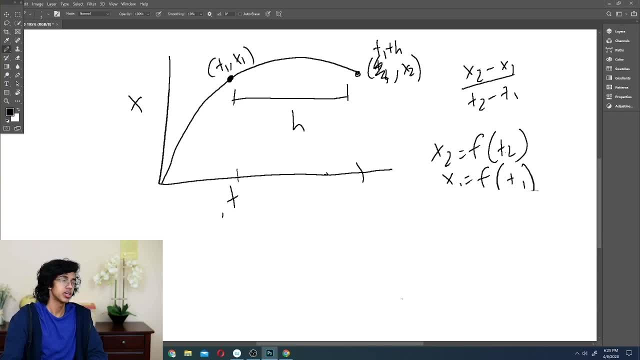 Then this is going to be t1 plus h. And then what's x2 going to be? It's going to be f of t1 plus h. Wowio, Now we can apply the same formula. okay, So we have f of t1 plus h, minus f of t1, and then over h, because h is the delta x. 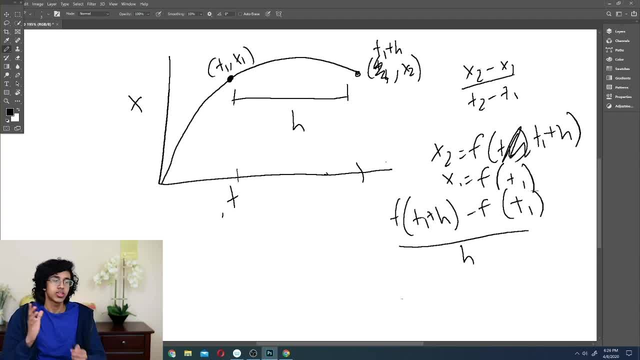 Epic. Now, in order to find the derivative, we want to make them as close as possible to each other, and that happens as h approaches 0, because h is the distance between them. So we can basically take the limit as h approaches 0.. 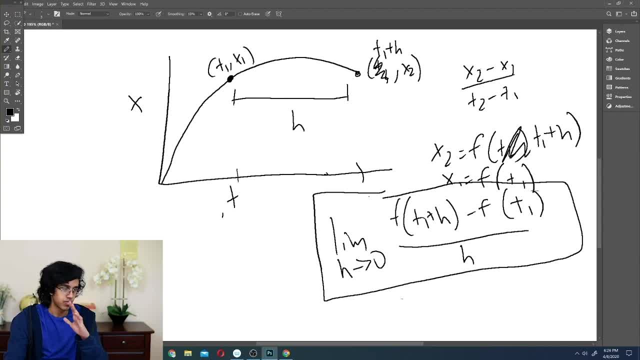 So this is the other definition. So now let me give you a tough version of this and let us see whether you can figure it out. So let us say it's asking us to find the limit, as h approaches 0 of f of t1 plus 2h minus f of t1 over h. 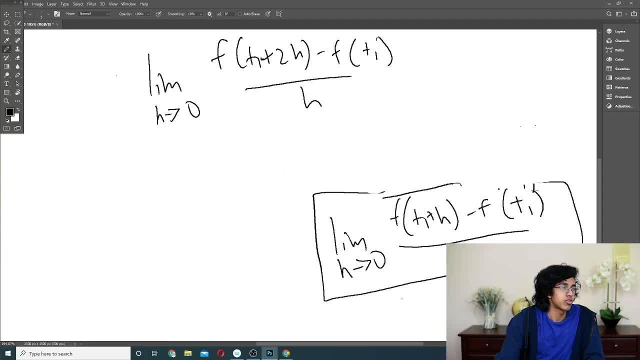 And it wants us to find this in terms of the derivative of f. Now, like, the way I like to think about these kind of problems is like: these are the two x-coordinates, right, And then the f of those are the two y-coordinates. 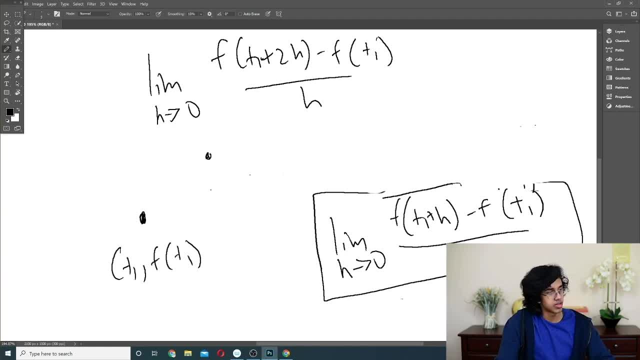 So we got the point t1, comma f of t1.. And then we have the other point, which is just t1 plus 2h, comma f of t1 plus 2h, And basically what the limit of h approaches 0 is doing. is it basically bringing these points infinitely close together? 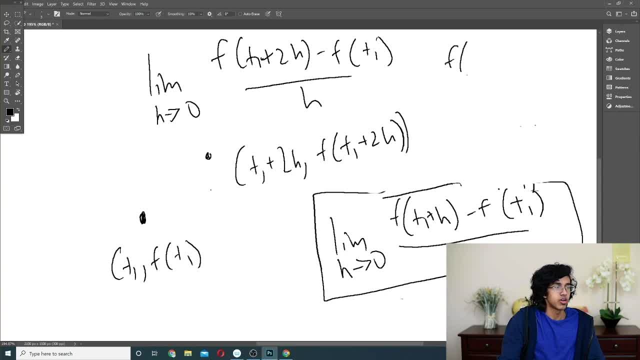 So what is the slope? in this case It's going to be f of t1 plus 2h, which is a y, And then we want to find delta y, so we subtract the other y And then we have the derivative. 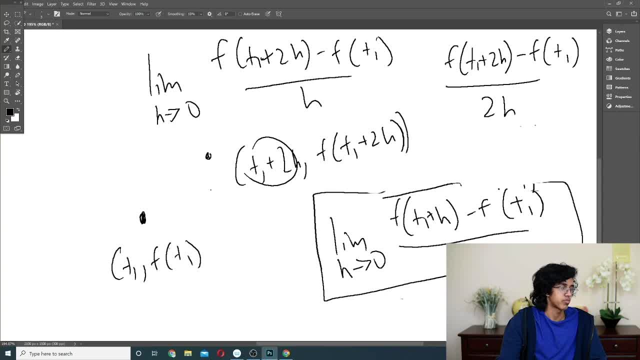 We have delta x, which is going to be just 2h, because this x minus this x gives you 2h. So this over here is equal to f prime of t1.. So then, if we want to find this, how do we get from this over here to that? 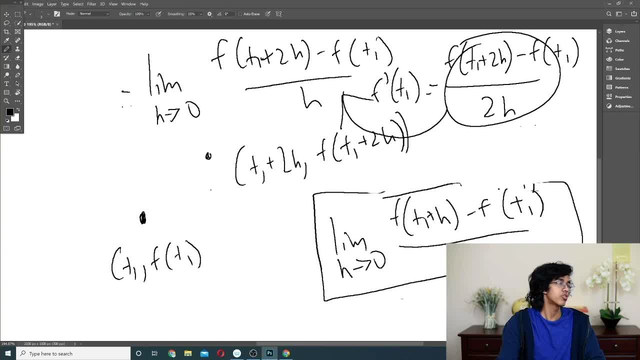 We have to multiply by 2. That is right. So this over here is just equal to 2f prime of t1.. So the best way to do these problems is literally just find the slope of the two points by using the numerator and then find a way to multiply that slope by to get the answer. 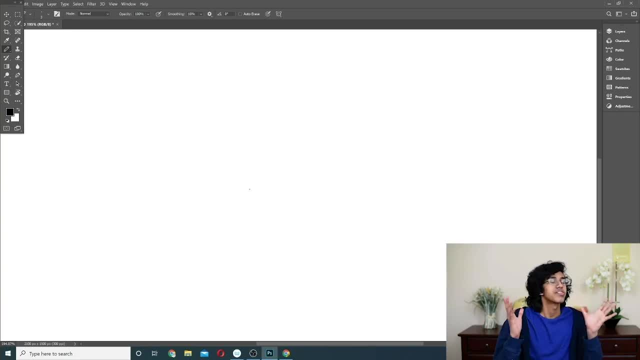 Dude. AP questions that use tables are so triggering because it's like: come on, just give us a function, that's math. okay, We don't need estimation nonsense. Well, fine, estimation is math. I don't like it. I don't like that nonsense. 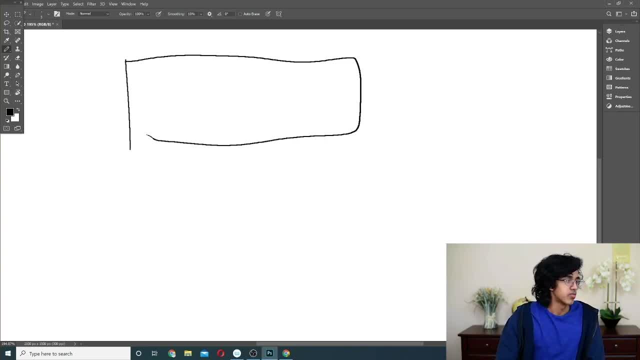 But let us do a table problem. So what they like to do is they like to give you an x and an f of x thingamajigger, and then they give you a couple points And then the question gives you this table and it's like: 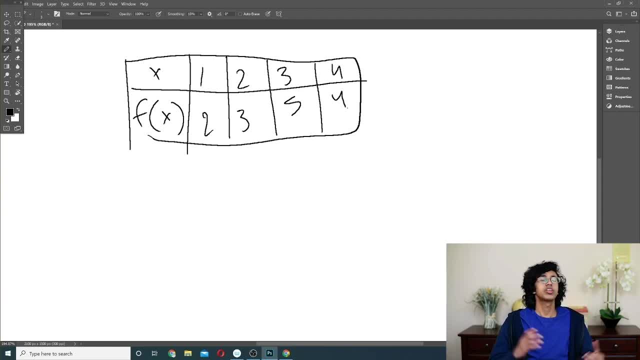 what is the tangent line at x is equal to 3? So this is going to be a double whammy. We're going to introduce two concepts at once. So in order to get the tangent line, you first got to know its slope. okay, 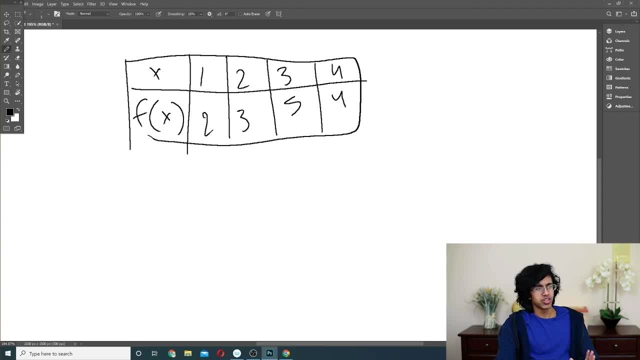 So the way you do that is, you take the point on the opposite side. okay, you don't use this guy, You use the opposite side of it. You don't use the actual thing, You use the sides of it. Just remember that. 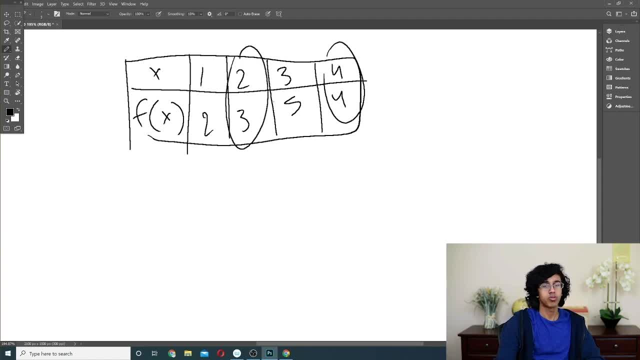 So we basically use the slope from this point to this point as a proxy for the derivative. So what's our delta y? f of x is our y, so it's 4 minus 3, which is 1, and then our delta x is 4 minus 2,, which is 2.. 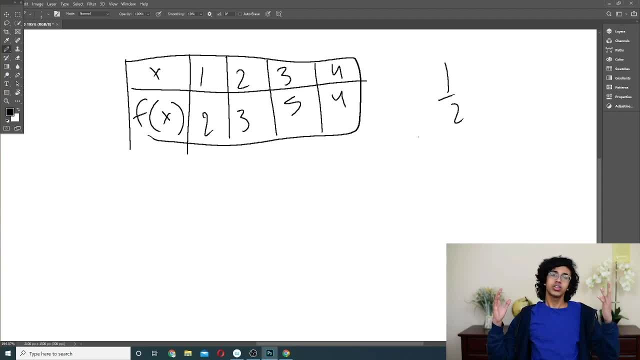 So we have a slope of 1 half for a tangent line. Now what are the two things you need in order to find a line? Two points, Okay, fine, we don't have two points, We have a slope, Come on. 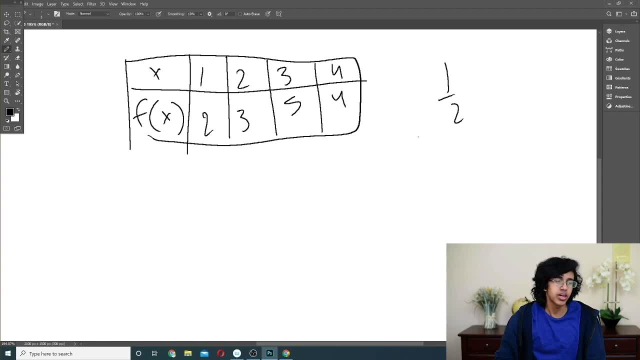 What else do you need? That's right, You need a point and a slope, And we could just use point-slope form and then solve for the equation of a line. So what point do we know is on the line? We know that it touches f of x at 3,. 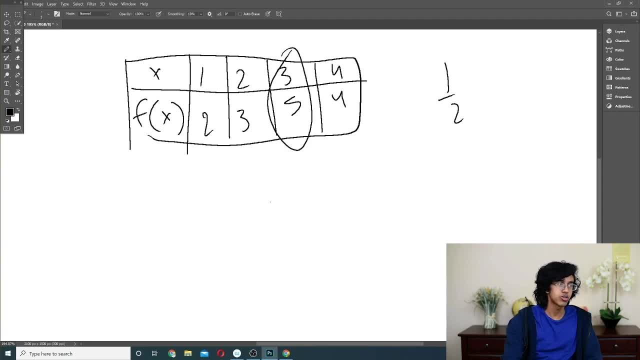 so that means this point has to be on both the line and the function. So we know that y minus 5 is equal to 1 half x minus 3 by using point-slope form with the point, And then we could just solve this for a cool epic slope-intercept equation. 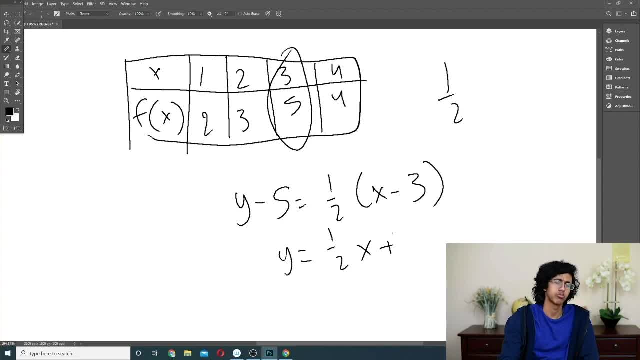 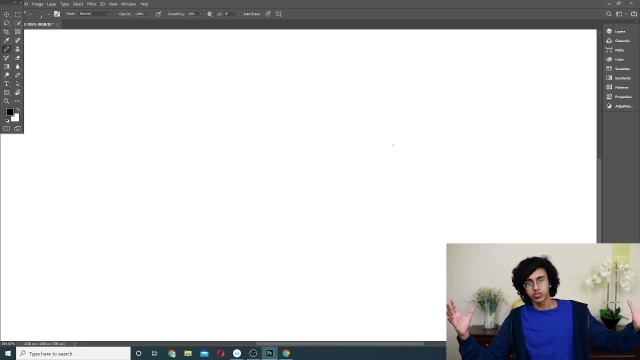 and we get: I can't math. How do you add 5 minus 3 over 2?? Oh, it's 7 over 2.. Very epic, We did it Nice. So now we've got to talk about the difference between differentiable and continuous. 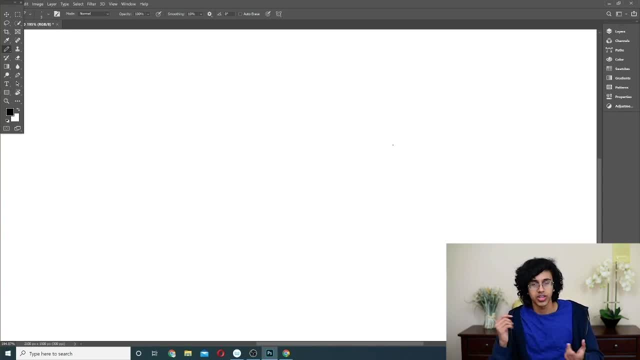 We already know what continuous is right. That's basically meaning that you can find the limit at any point. Let me just rewrite the thing. So we've got. continuous is basically lim as x approaches c of f of x is equal to f of c. 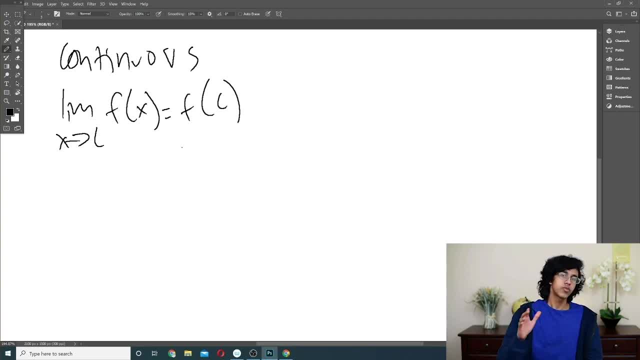 And this is true for all points in the interval you want to prove as continuous. Differentiability, however, is very different. Differentiability is that you can find the derivative at a certain point, which makes sense. right Differentiability: able to differentiate. 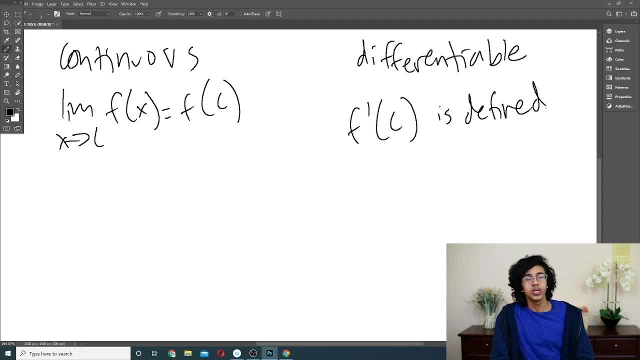 Like I mean, it's not that complicated. So basically there are two corollaries between the two things And like the proof is not very interesting, but like the common sense makes it a lot easier to remember. 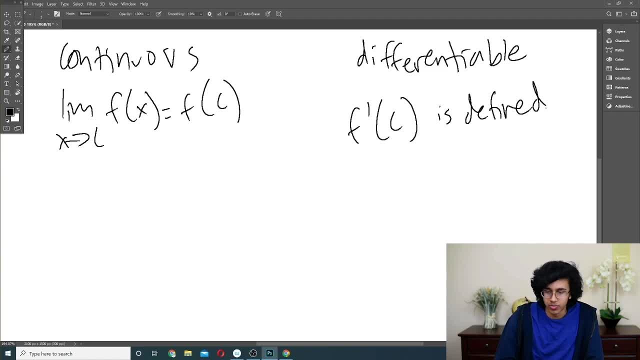 So the first thing is, let's say that a function is differentiable, right, You can find the derivative, Then you know that it's continuous, Because differentiable means like you're at a point right, And it has a certain slope. 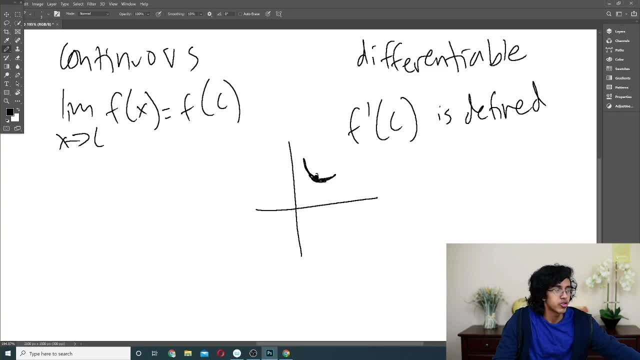 So it must like come out on both sides, right? So like if you know that it's differentiable, it's like coming out from both sides, So this looks continuous, This is continuous. So it makes sense that if it's differentiable, it's continuous. 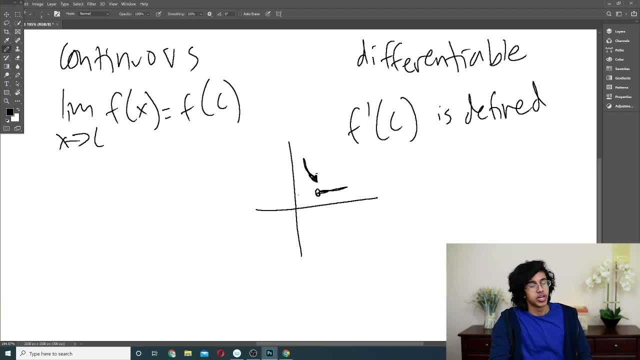 Now, if it's not continuous, how is this differentiable? It can't be. It doesn't make any sense, Like the derivative here is different from the derivative here. What So? the other thing is that if not continuous, it can't be differentiated. 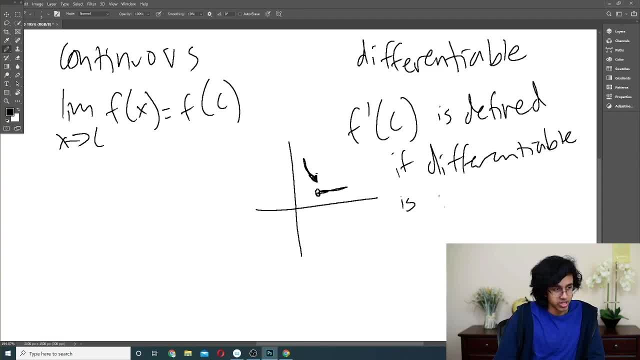 Let's write it out. So we got: if differentiable is continuous, And then we also got: if not continuous, then not differentiable. Very cool. I'll give a couple more examples so it's more clear why these make sense. But like, I just gave like a very basic logic, right there. 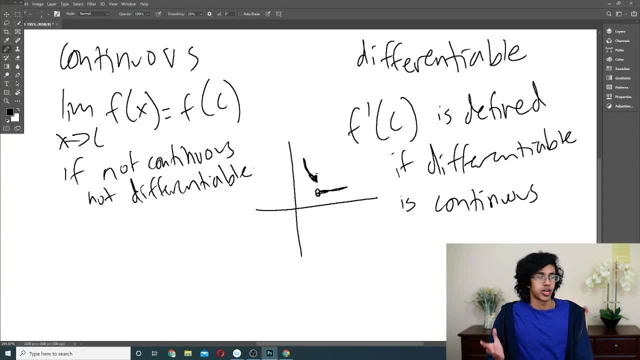 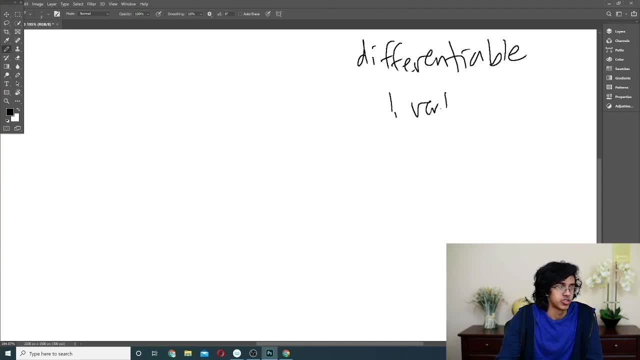 So now let's figure out how to determine whether something is differentiable. okay, So basically, there's only three ways that a function can't be differentiable. So the first version is that you have a vertical tangent. okay, So let's say you have a graph and it goes like this, and then it goes like that, and then it goes like that. 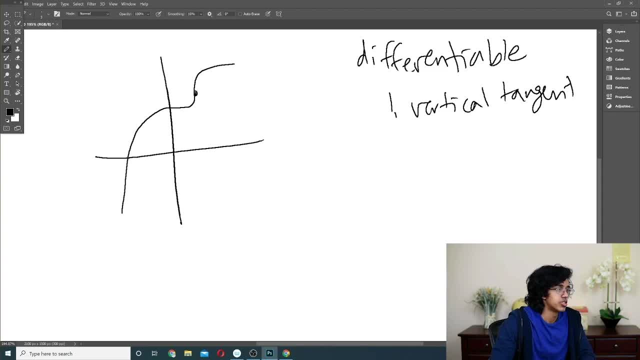 Well, blammo, Okay. so if I ask you for the derivative right here, the slope of the tangent line is like right, like that. And could I give you the slope of a vertical line? No, it's like infinite. 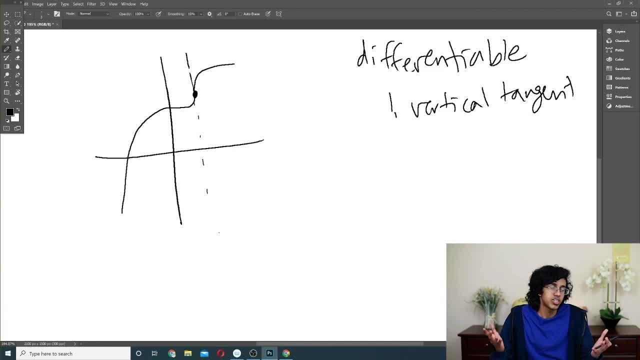 So you can't give a derivative there. so it's not differentiable. It makes sense. And then the second condition for which it's not differentiable is if it's not continuous, which we already explained. But just to give an example, let us say that like you got a random jump discontinuity here instead. 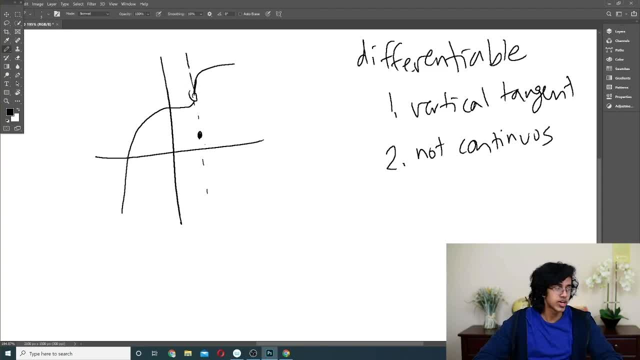 Oh, no removable discontinuity. I gotta remember my vocab. Don't worry, I know the calc I swear. So let us say we try to find the derivative right, Like if we did our normal formula, we would do lim as f of x plus h. 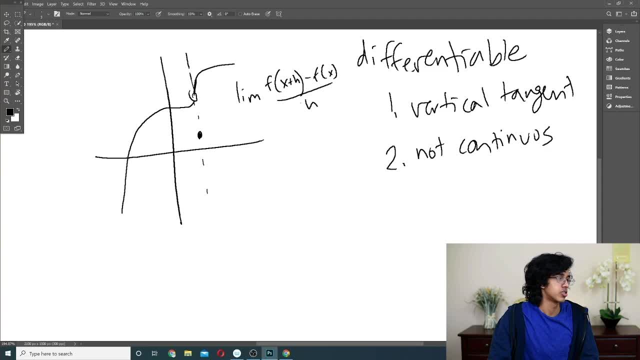 and then we did minus f of x over h as h approaches 0. So basically then you'd be trying to find the derivative like this and then like that and like that, And you can see that as it approaches here. 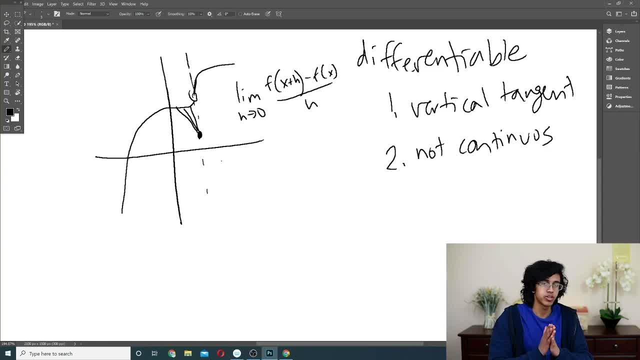 this line is getting steeper and steeper as your h becomes 0. And eventually it'll be straight up. So, like this doesn't make any sense, Your derivative is going to be infinity, but it's clearly not defined. 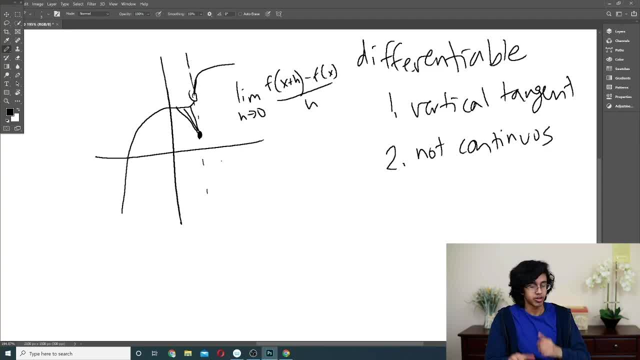 It doesn't make any sense whatsoever that we're taking the derivative even here, Like: how is this over here? a tangent line? This one doesn't make any sense. So if it's not continuous, you can't differentiate it. okay, Keep that in your head. 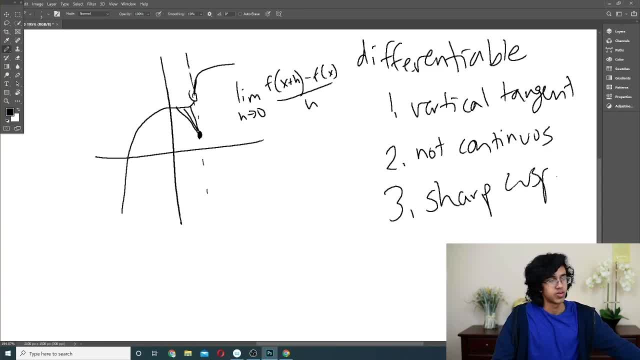 And that's it. And then the third one is the coolest one. It's a sharp cusp. Actually that's kind of redundant Just say cusp. you know what? I know how to English, okay, I swear. And basically a good example of this is: if you have like that, 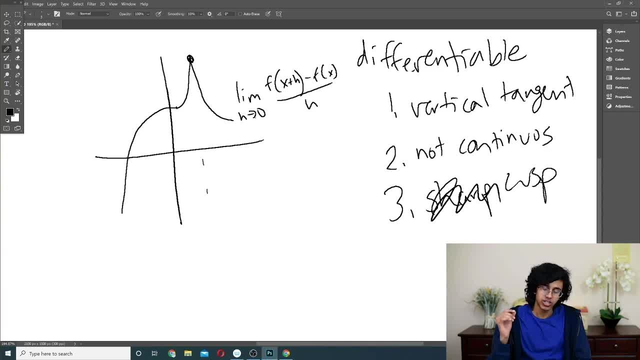 So let's think about derivative as a limit. right In a limit. we already explained extremely clearly that your limit has to approach the same number if you come from the right and if you come from the left. But in this case, your derivative as you approach from the right is going to be this way. 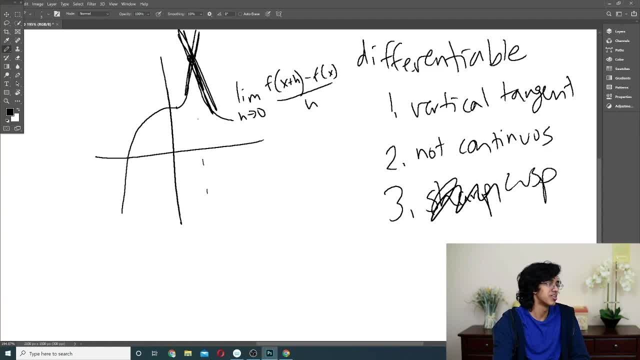 Like what the heck? And then if you go from the other way, it's going to be that way. No, This is not okay. okay, Do I have a limit approaching two different numbers and expect us to give an answer? No, 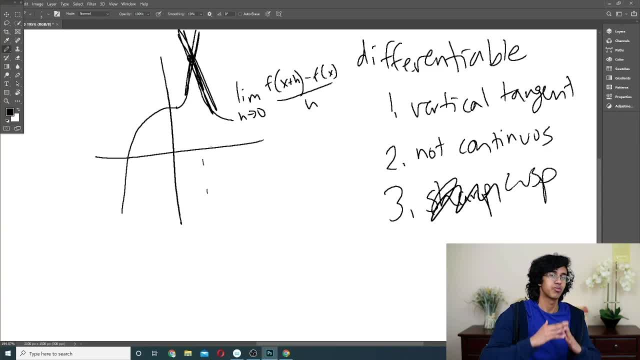 So it's not differentiable at a point where the derivative changes. at that point I mean, of course, yeah, derivative could change, But it shouldn't be like an abrupt change, like a sharp point. Okay, so basically just remember these three things. 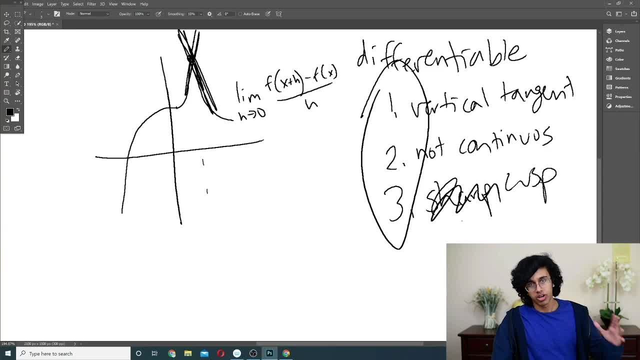 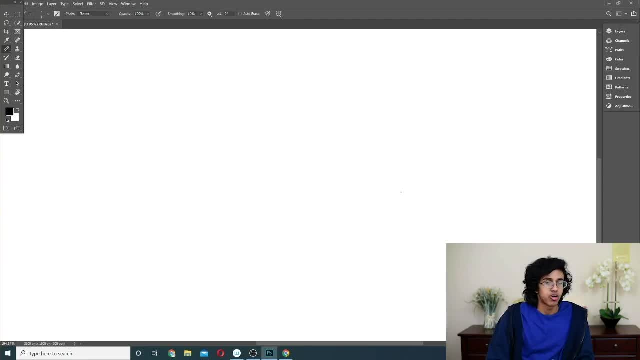 Vertical, tangent, non-continuous or cusp. Those are the three places where it's not differentiable. Okay, I don't know whether they'll ask this on the AP exam, but like I was looking at Khan Academy and they gave examples of how you solve limits without using limit. 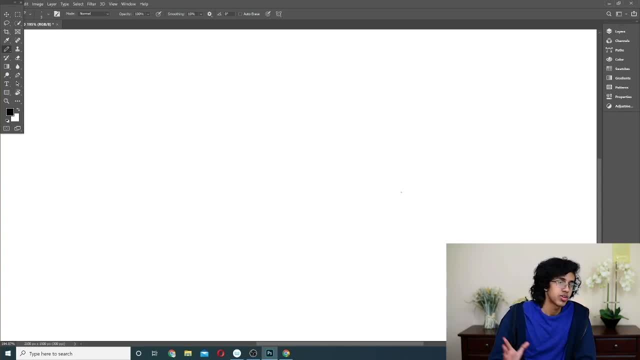 I don't know whether this will be on this year's AP exam, but like Khan Academy was covering, like how you could solve limits without actually knowing any of the rules, just by using the formal definition. So I'm just going to do a quick example here. 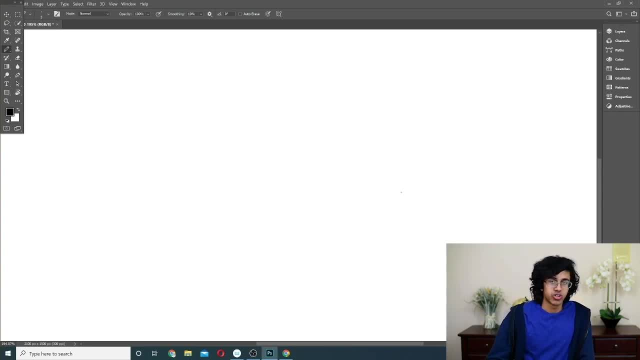 But if this ever comes up on the AP exam, just make sure to check your answers with all the other derivative rules that you know. So let's say it asks you to find the derivative of x squared at like any point. Let's say 8.. 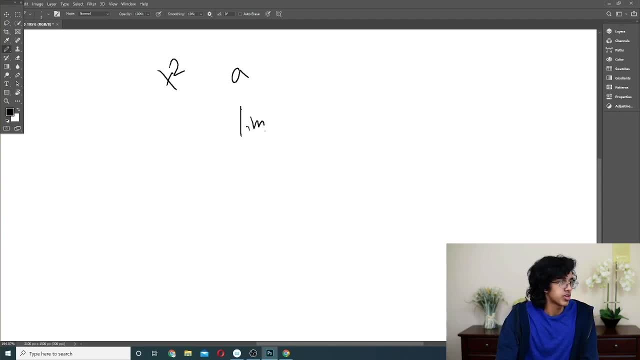 So if we think about our formal definition of a derivative, it's basically limit. h approaches 0 of f of x plus h minus f of x over h And f of x is equal to x squared. Wait, sorry, not x. This should be a. 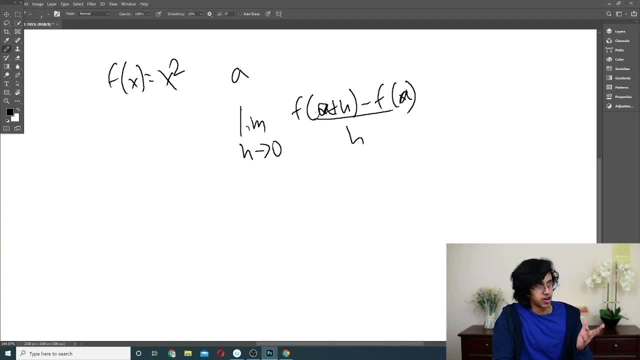 So that is the point at which we want to differentiate. So basically we plug in f of a plus h and we get a squared plus 2ah plus h squared. I basically just expanded out the squared version and then you subtract a squared over h. 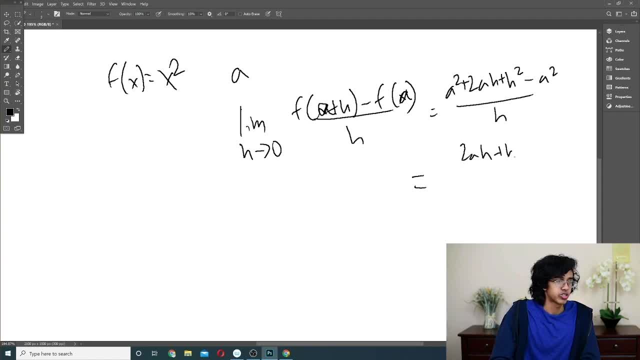 So this is just equal to 2ah plus h squared over h, And then this is equal to 2a plus h, And then h approaches 0.. So this is equal to 2a. Wow, Epic. So at point a, your derivative is just going to be 2a. 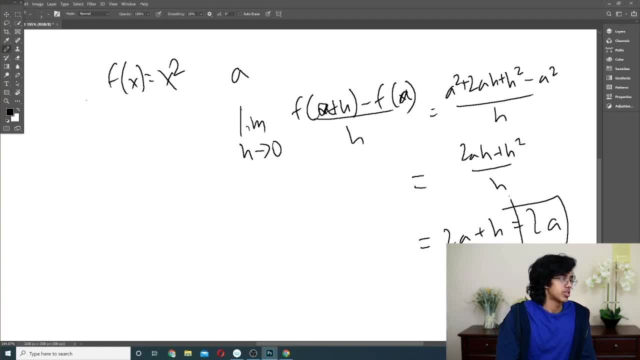 for x squared, Or in other words, you could write this as f prime of x is equal to 2x. OK, So that was kind of yucky. You don't want to do that for every function, And this is not even practical for every function. 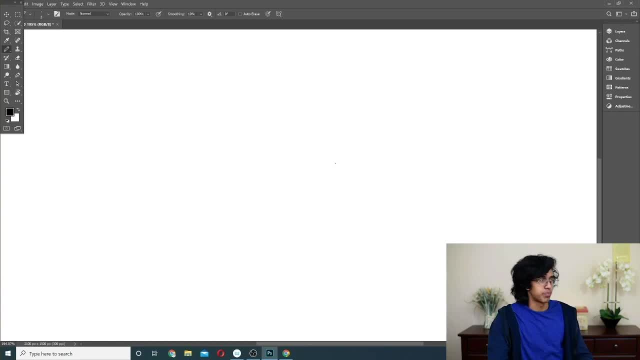 So let us learn the derivative rule. All right, First up, we've got the power rule. OK, And honestly this rule is not very powerful at all, but it's called the power rule, I don't know why. So if you have f of x is equal to x to the n. 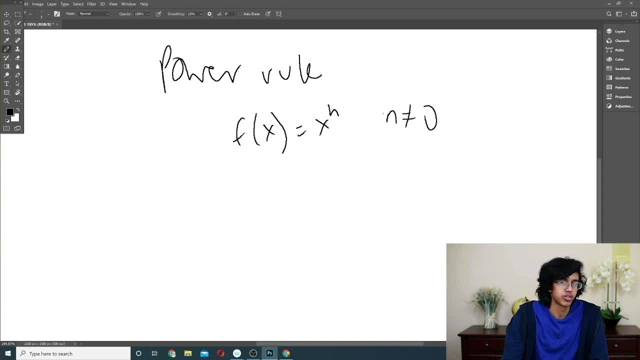 where n is not equal to 0, because if you have n is equal to 0, you have a constant, because x to 0 is 1. And the derivative of a constant is always 0. Because if you look at a graph right, 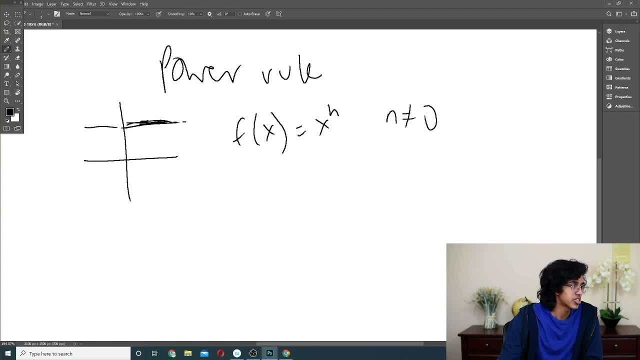 I mean a constant just looks like that. What's the rate of change in this? It's just 0.. That is right. It doesn't change ever. It's called a constant. That's why it has a derivative of 0.. 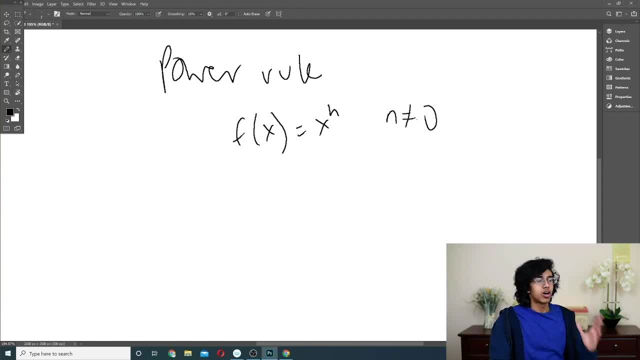 OK, I should stop, But anyway. the point is, when n is not equal to 0,, if we take the derivative of this function, we basically get n times x to the n minus 1.. Explaining this for positive integers is basically just what we did for x squared. 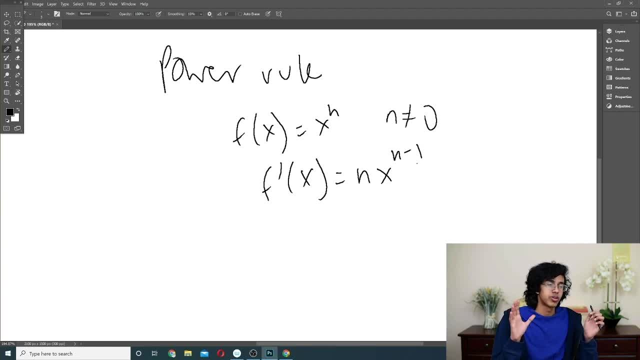 but for other stuff it's kind of hard, so we're just not even going to worry about it. Maybe we probably won't even mention it. So basically, for example, the derivative of x to the 6th is going to be 6x to the 5th. 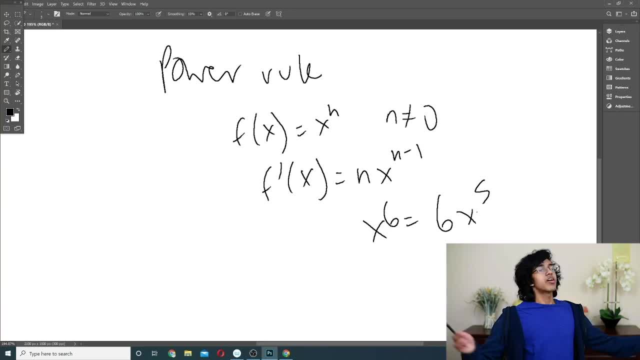 You guys know how to plug in formulas. You better, OK, You better, But we have more interesting rules to talk about. OK, So let's talk about the other properties. All right, so we basically already talked about how, if you have a constant, 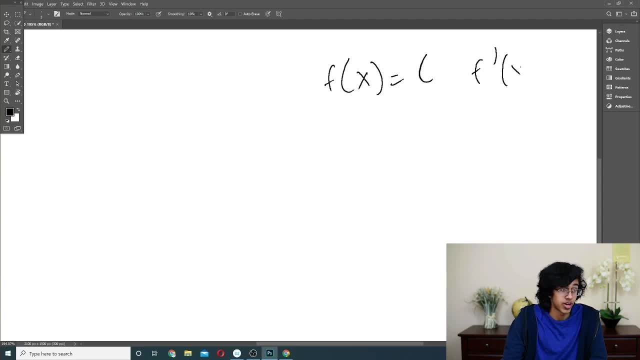 f of x equals a constant, then we basically have f. prime of x is equal to 0.. Another cool thing about differentiation is that you ignore addition signs. basically They just go through as if they were not affected at all by the thing. 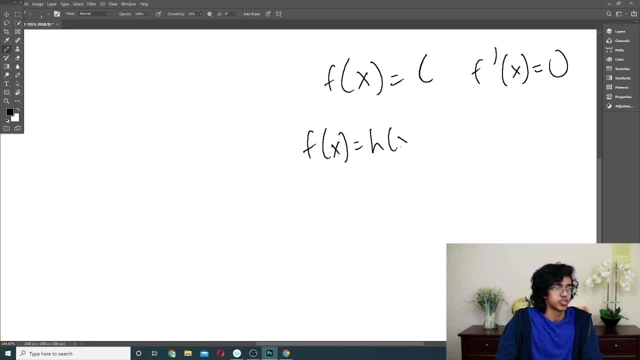 So if you had f of x is equal to 0, h of x plus g of x, then we basically have f prime of x is equal to h prime of x plus g prime of x. In essence, you just take the derivative of the individual parts that are being summed. 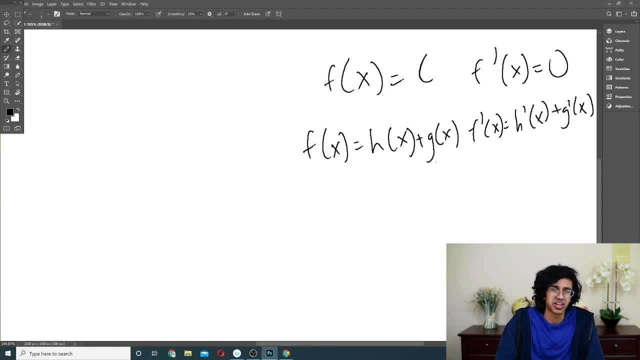 and just sum them at the end. OK, difference is just applying the negative version of this, so it's not that complicated. And then the last thing is if you multiply by a constant. So let's say f of x is equal to k times g of x. 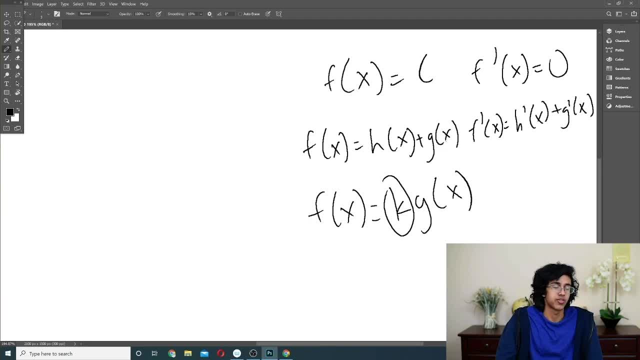 Basically this thing in the front, the coefficient just doesn't get affected. So you could literally ignore coefficients. So it becomes k times g prime of x. OK, now, these are pretty common sense. You should probably know these if you've taken any calc at all. 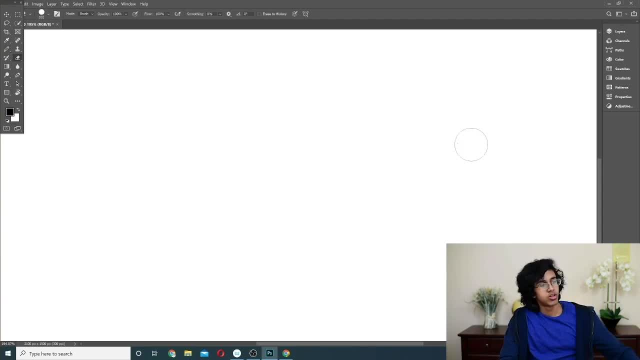 So it should be Gucci. So now let us see what we can do. So there's one type of annoying problem. they like to do about these really simple derivative rules, and they like to give you a table and then they ask a question about it. 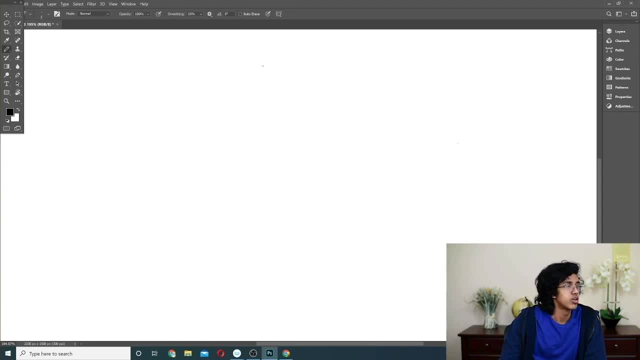 So why don't we combine two things into one? OK, so let us first combine our power rule into this. So let's say we have: f of x is equal to like x cubed plus 3x minus 2.. OK, and then we have g of x defined by a table. 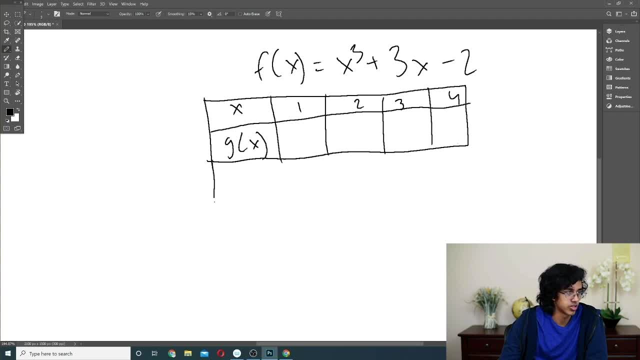 And we are going to: oh, and then it also gives you the g prime of x, And then I'll just fill this in with arbitrary numbers, As you can tell, very arbitrary, And you can guess which number we're going to take: the derivative right. 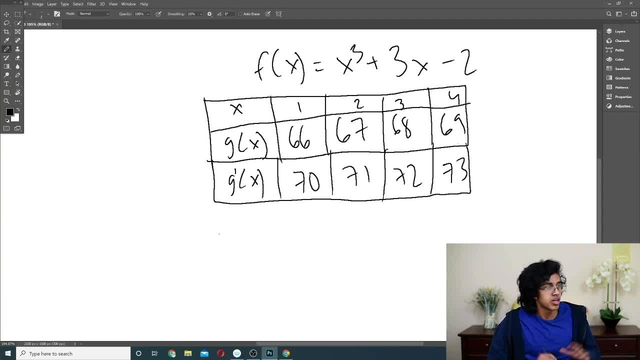 But first we can't get too excited about using the number 69. We first got to define what the function we're taking the derivative of is. So let us say that h of x is equal to f of x plus 5g of x. 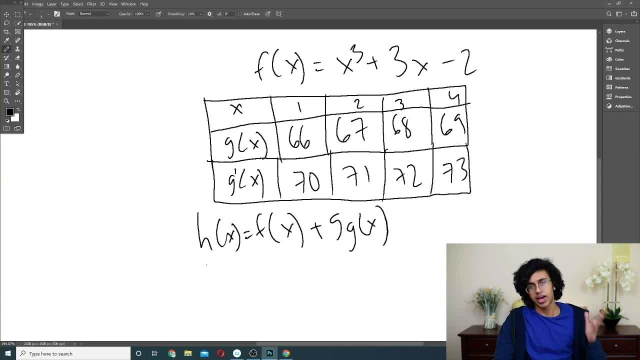 Then it's asking us what is the derivative of h of x, h of x at 4.. So first we just derive this right, We get h prime of x is equal to f prime of x plus 5g prime of x. 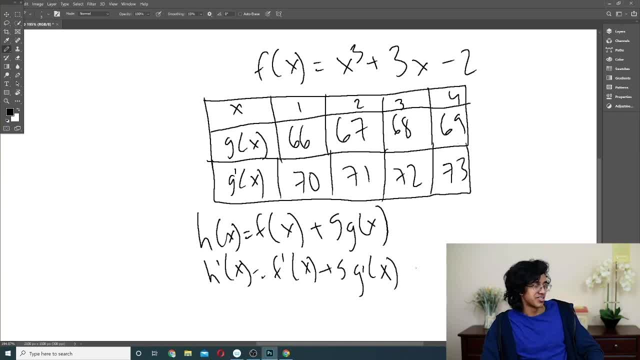 No, god dang it. 69 is not you. This is so sad. I tried so hard, God dang it, But anyways. so in order to define this, we first got to take the derivative of f of x. So f prime of x in this case is going to be equal to. 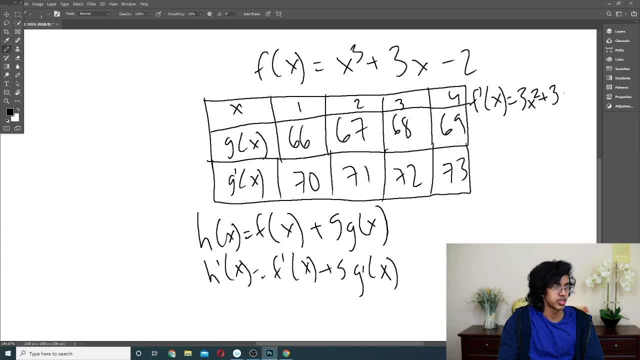 using power rule on the first one, 3x squared. Using power rule on the next one, 3 minus 0.. So if we plug in 4 to this, we get f prime of 4 is equal to what 4 squared is: 16,, 48,, 51.. 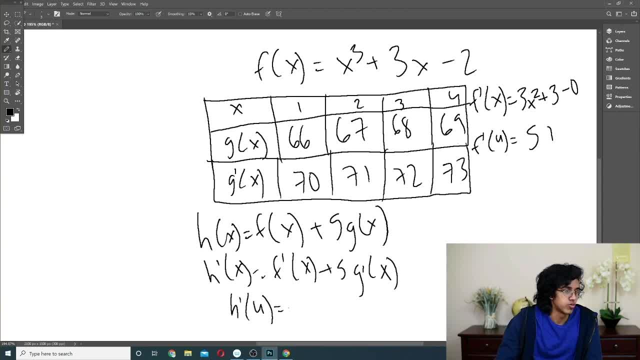 Okay, So h prime of 4 is equal to 51, plus 5 times g prime of x, which is 73. And this I should not have chose such a big number. Now you guys got to make a fool of me doing math in my head. 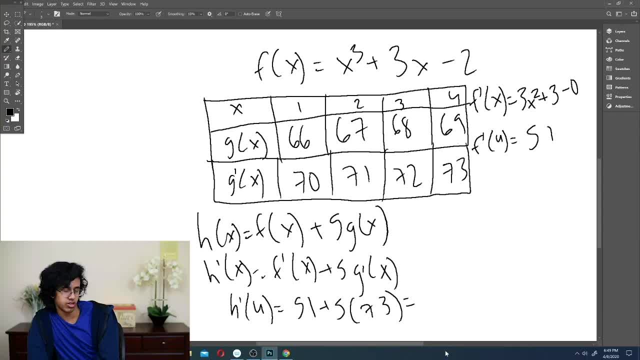 350 plus 5,, 365 plus- uh, Okay, 4, 16.. God dang it. Why do I do this to myself? Okay, That's out of the way. Let us figure out some more rules, All righty. 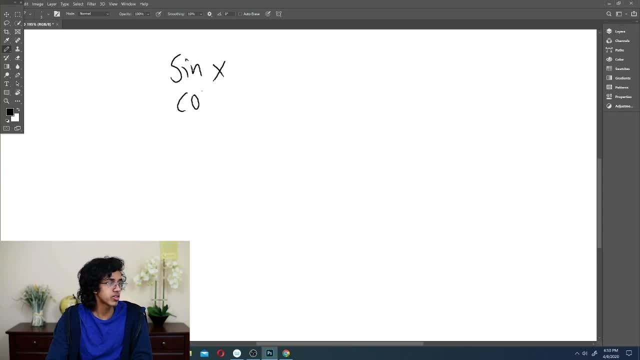 What is the derivative of sine x and cosine x? That is your next question. I bet you guys were thinking that the whole time we were doing this video. Basically, I'm just going to tell you because I'm a meanie. So we do d over dx and we do d over dx. 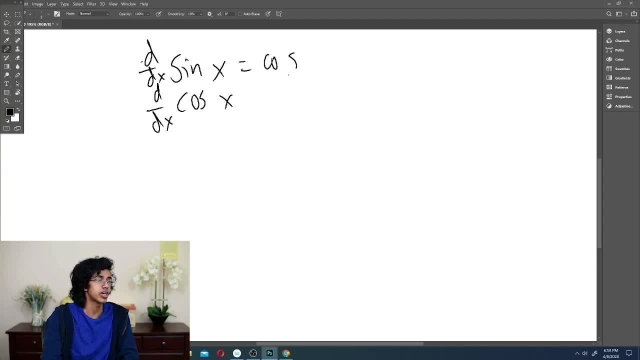 You basically get: this is equal to cosine x and this is equal to negative sine x. Now I know this trips up a ton of people Like: where do you put the negative sine? Where do you put the sine x? Where do you put the cosine x? 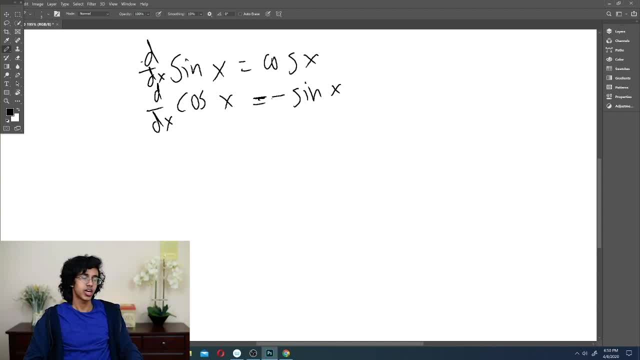 This is just a bunch of jumble of negative sines and cosines and sines. What the heck So like? the easiest way to remember it is to just look at a graph. So like, if you don't want to look at a graph, 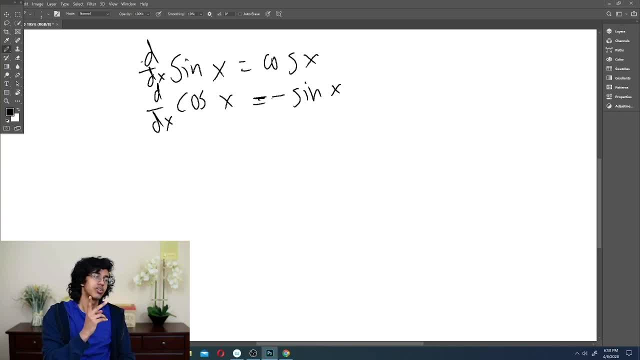 like. the fastest way to do it is: just know it's flipped and then like: sine goes to cosine, cosine goes to sine, and then like: whenever it starts with a, c, the derivative is negative. This applies to like, cotangent and cosecant. So it's a really useful thing to remember. 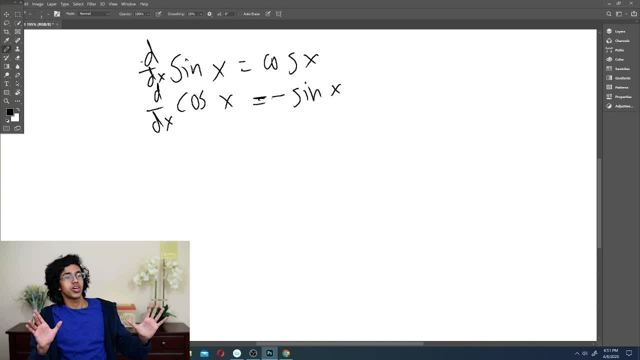 If it starts with c it's negative. But if ever in the test you forget, if ever you want to just make sure that you got the right sine and you got the right full function, you can just draw the graph okay. So let's look at a sine graph, right? 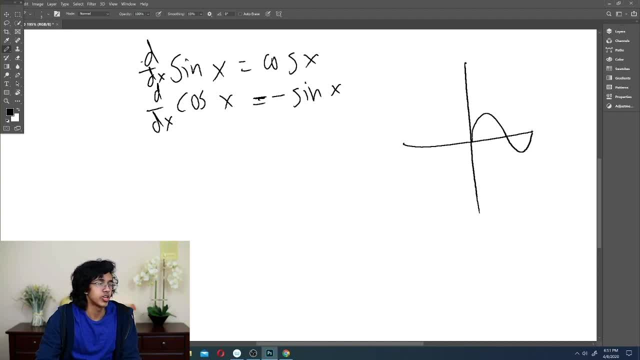 Starts at zero. It goes like that: Okay, So over here, right, it has a positive derivative, And then over here it has a zero derivative. So if you're trying to put sine x right at pi over two, 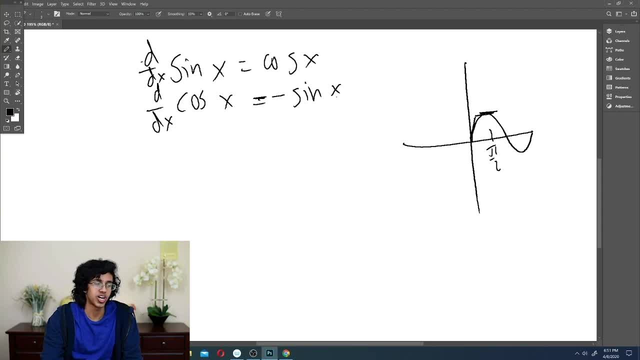 the derivative should be zero. But if you plug in pi over two to sine x it would give you one. So sine x, the derivative of sine x, just can't be sine x, because then it would give the wrong value, And cosine x works perfectly. 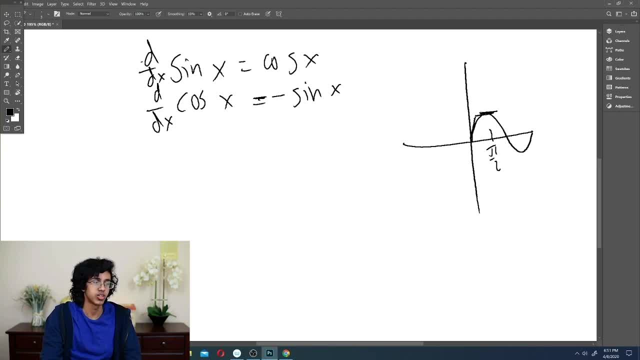 because it has a positive one. slope over here and it goes to zero at pi over two Makes sense Also because it's positive. you don't want to put a negative sine in front of the cosine, because then it would be negative and that just doesn't make any sense whatsoever. 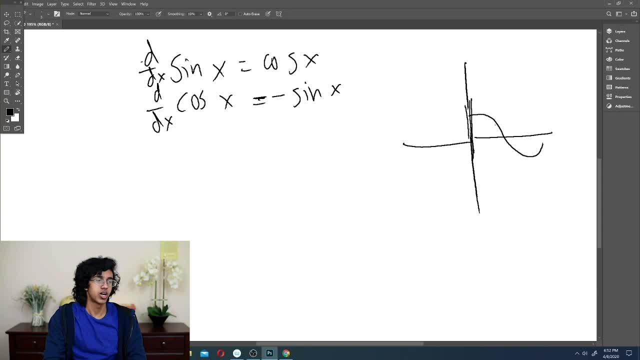 Okay, Let's look at cosine. It's like this: right Starts off zero and it becomes more negative as time goes on. Same with sine Negative: sine x starts at zero and it becomes more negative. So it makes sense that it's going to be the derivative of cosine x. 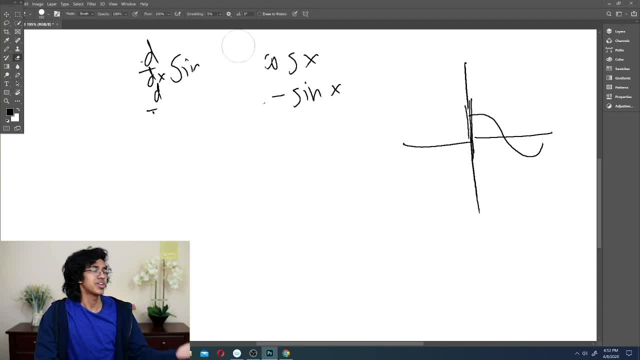 Very cool. All right, That's a cool trick. Just know it. I mean, you're probably going to be able to remember that derivative of sine x is cosine x and derivative of cosine x is negative sine x. You better remember that, okay. 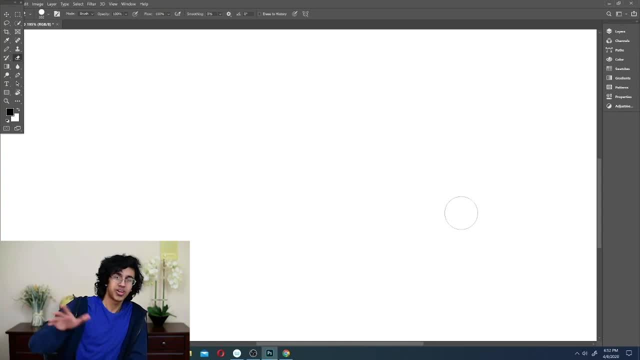 That is important, But you know, if you ever need it, it also applies to everything else, so it's a good trick. Okay, Derivative of e to the x is just equal to e to the x. I don't know how else to remember that. 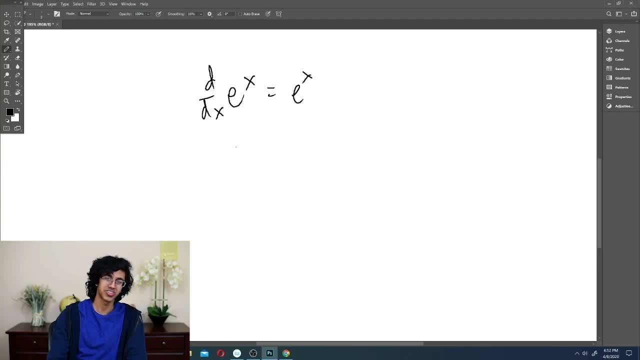 If you can't remember this, then you might as well just not take the test. okay, And then the derivative of ln of x is equal to one over x. Very cool, I don't know, Somehow the way I remember it is like. ln x seems like. 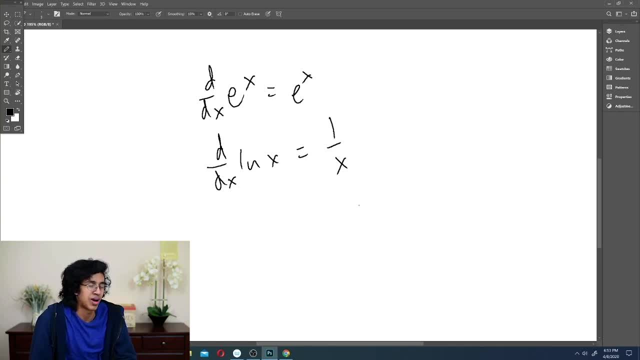 you're telling x to go down somehow. I don't know how that got into my head, but I don't know. That's just how I remember it. ln x: I don't know, Maybe I'm just too used to telling ln to go under. 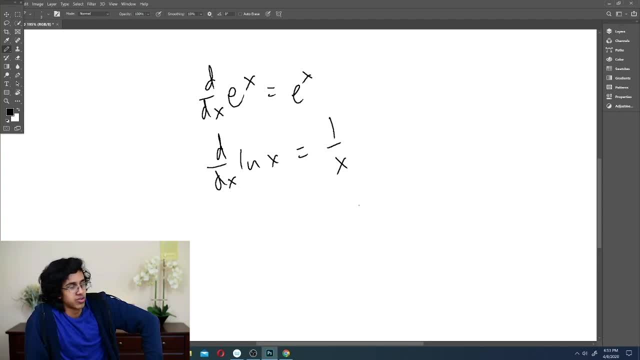 Okay, that's weird, Fuck. Anyways, the point is derivative of ln. x is one over x- More rules. okay, We need more rules. We are hungry for rules, We are thirsty for rules. Let's keep going. Product rule. 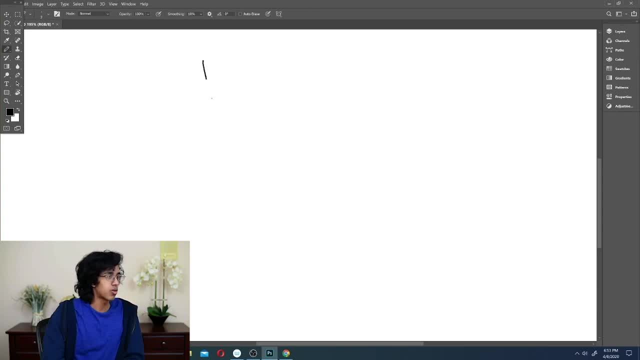 Okay, so basically, if you have, h of x is equal to f of x times g of x, h prime of x is equal to f of x, g prime of x plus f prime of x times g of x, times g of x, x g of x. 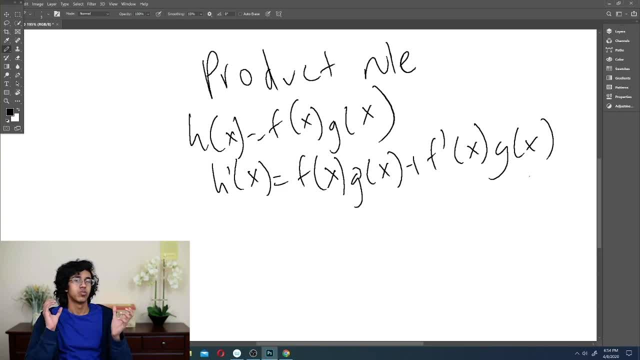 Okay, this one is really easy to remember. Just remember that like one derivative paired with the other non derivative, and then just You just have to get all the combinations out there And then the last rule is kind of yucky, like very yucky. 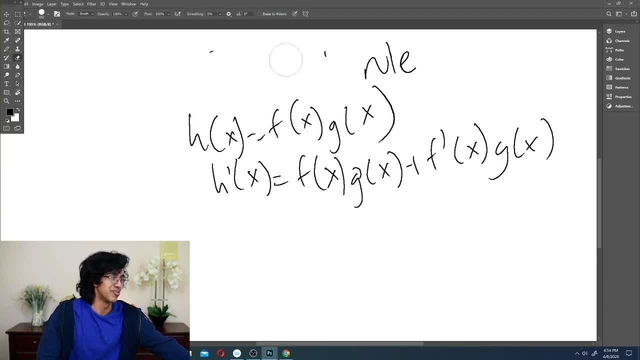 Like I don't even like remembering it, so I just re-derive it every time, But it's called the quotient rule. So you have: h of x is equal to f of x. everybody over. g of x is a new rule, Aw. 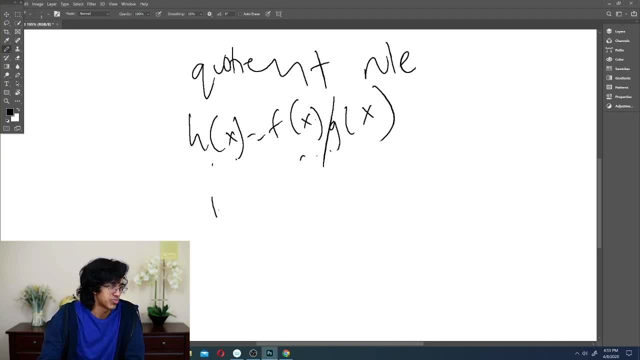 do I even remember it? Okay, low d high, high d low is equal to low d high, so low, which is g of x times d of high minus. uh, this is so hard: f of x, g, prime of x over g of x squared. but this is just so hard to remember i keep forgetting it. 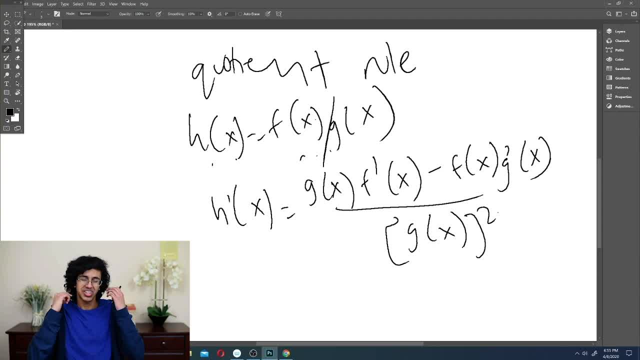 was high d low, low d high or low d high, high d low. i just that thing doesn't stick in my head. but if it worked for you- low d high, high d low- just remember that. but i'm just going to derive it because that's how i like to remember it. just use the product rule, okay, so like you know that, 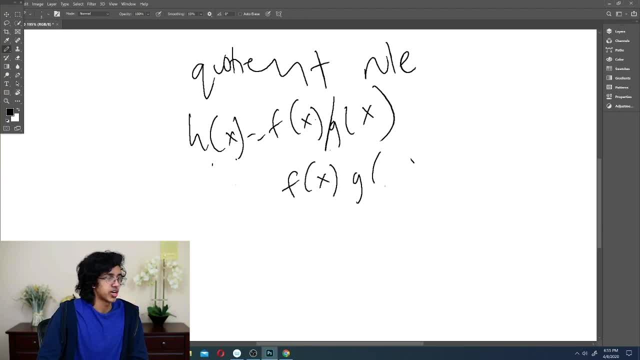 um, this is basically f of x times g of x to the negative one. okay, well, oh, do we even learn chain rule? god dang, we don't learn chain rule in this unit. god dang it chain rule. then the other unit? i can't use this derivation then well, who cares? you guys probably know the chain, i'm just going. 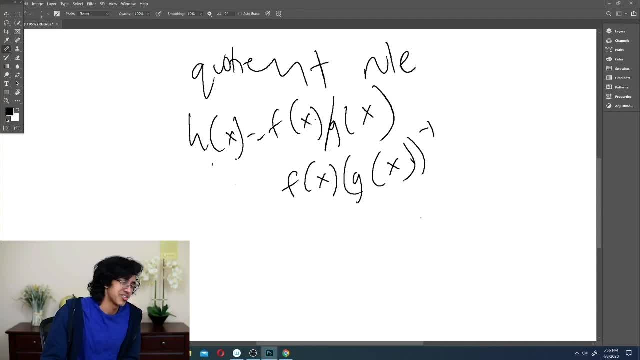 to explain the derivation quickly and if you don't understand it, just wait till the next video. so if you take h, prime of x is basically going to be f, prime of x, time one over g of x, plus the derivative of this part, which by the chain rule is going to be negative, of g, prime of x over g of x. 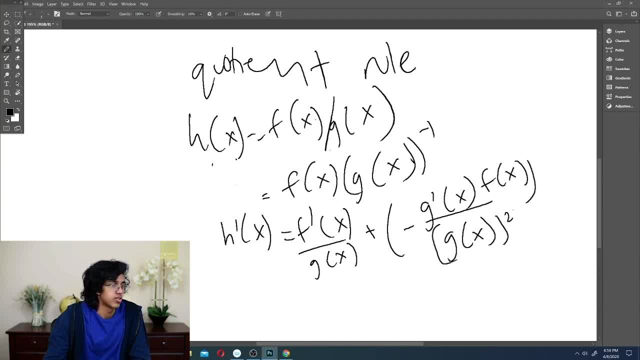 squared times f of x. and then if you do out the math, you basically get that f prime of g of x- what whoops? f of x times g of x minus g. prime of x times f of x over g of x squared. nice suit, good stuff, boys. and then, last but not least, we gotta remember the last. 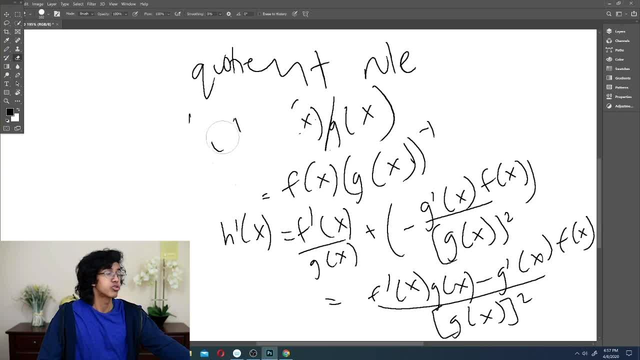 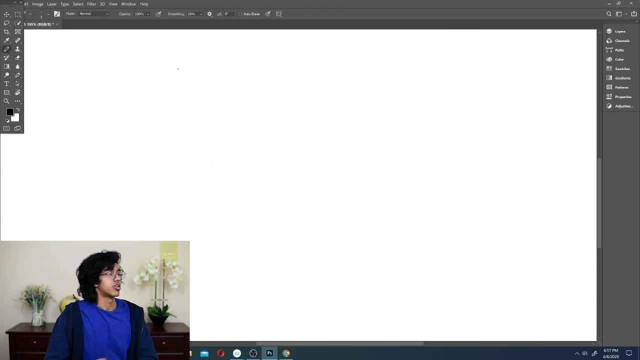 of the trigonometric, trigonometric. there we go, we got it, we got it. we got it boys. oh, i didn't even finish the sentence. trigonometric functions. that's why we gotta finish. so we got our sine x, we got our cosine x. well, that's lame, we need more. so we got tan x, we got cotangent. 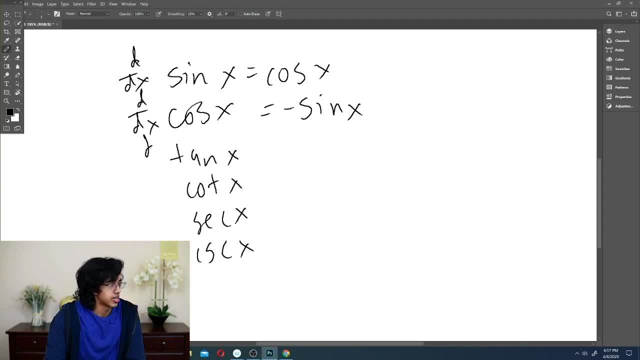 x and we got secant x and we got cosecant x and we gotta take the dx out of all of these boys. alright, epic. so basically, tan x is just secant squared times. g of x over g of x over x. cotangent is negative cosecant squared x, secant is. don't expose me. secant x, tan x. 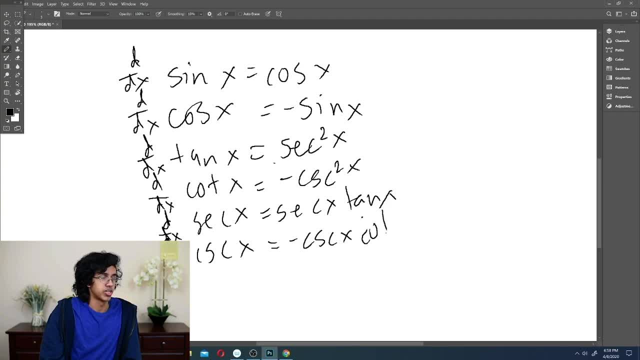 and then this one is equal to negative: cosecant x, cotangent x. okay, now, like this is not the easiest thing to remember, but like the one that you for sure have to remember, that i don't really have a way of helping you with is this one. and this one like the way i like.